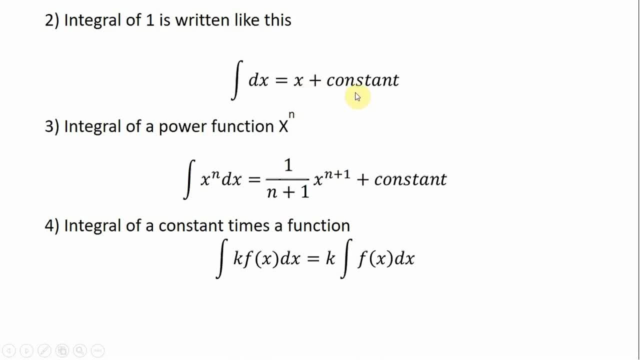 can check our answer. if we take the derivative of x plus a constant, what do you get? The derivative of x is 1.. of a constant is 0, so we get back what we originally took: the integral of The important integral of a power function where x is raised to some power n. the rule is as follows: 1. 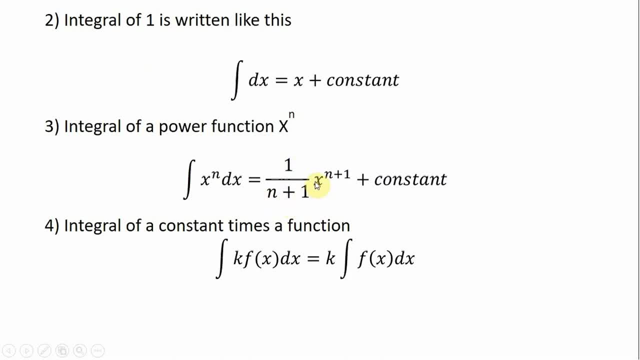 divided by n plus 1 is going to be multiplied by x, raised to the n plus 1 power, and again we add on some constant. So this is an important rule that we'll use in a little bit. And then integral of a constant times a function. what we can do is we can bring out the constant. 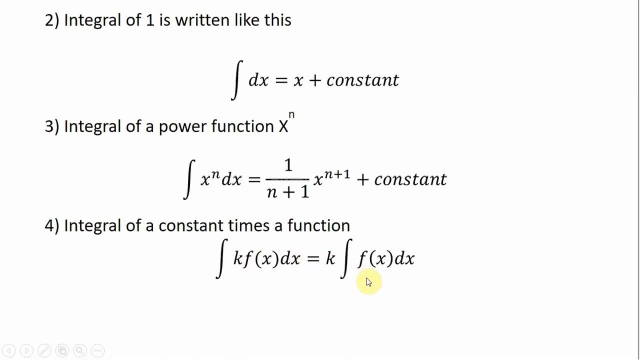 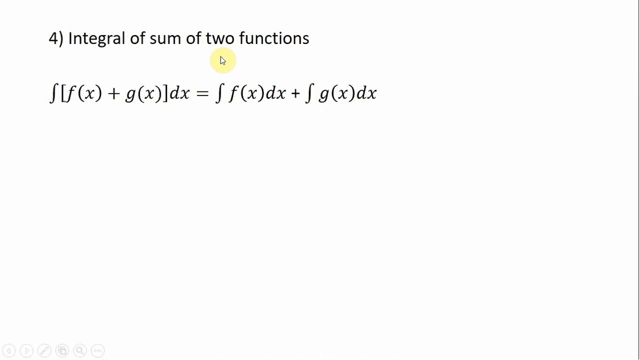 in front of the integral sign and then just take the integral of this function, f of x, and then multiply it back through by k, And finally an integral of sum of two functions, or it could be a, d. If there was a difference of two functions, this plus sign would be a minus sign, So we 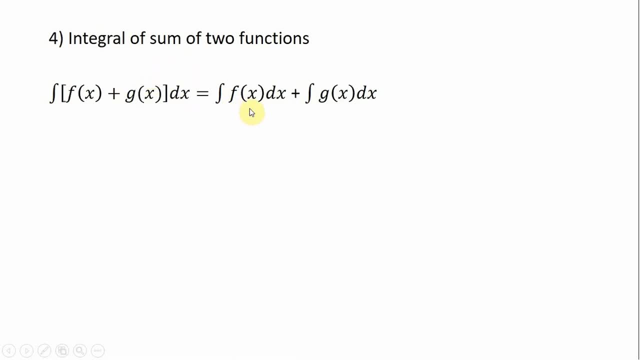 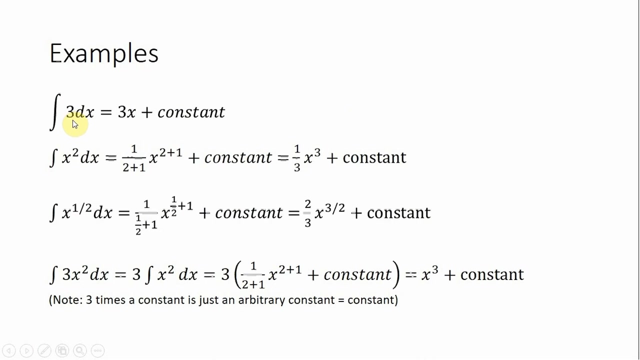 can break down the sum of two functions as follows: Take the integral of f of x, then add to it the integral of g of x. Here are a few numerical examples that apply some of those rules. The integral of 3 is just 3x plus a constant. Again, note: if we took the 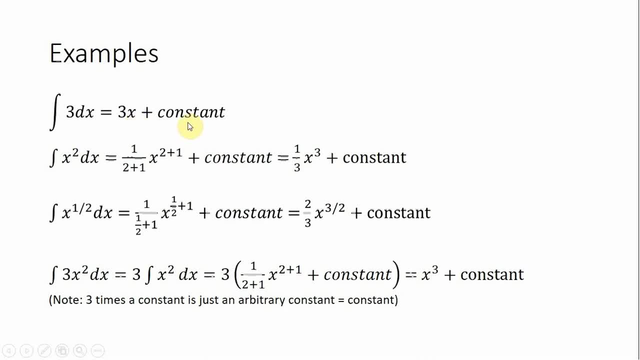 derivative of this answer, the derivative of 3x is 3,. the derivative of a constant is 0, so we just get back what we're taking: the integral of The integral of x squared. we're going to use that rule here. n is 2, so in the denominator we have n plus 1.. So since 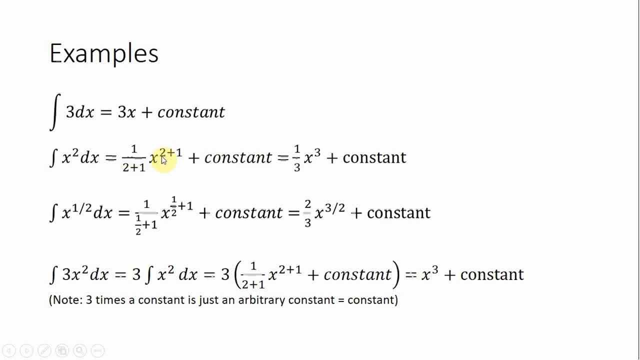 n is 2, we're going to have 3 down here And then, following that rule, again it's going to be x raised to n plus 1, where again n is 2.. So this will all simplify down to one-third: x raised to the third power plus a constant. 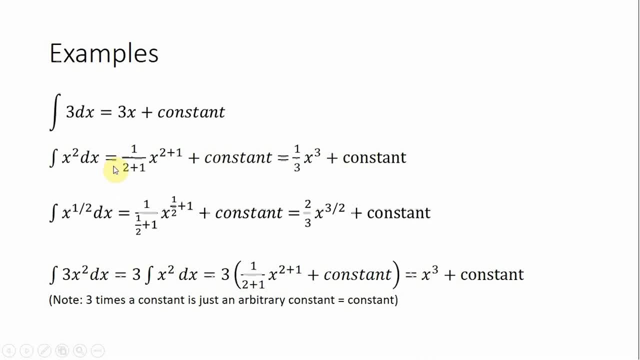 If you were to take the derivative of this result, you would get back x squared. Another example: here we got the square root of x, x raised to the power of one-half. Just following that rule, since n is one-half, it's going to be n plus 1 down here, And then x is going. 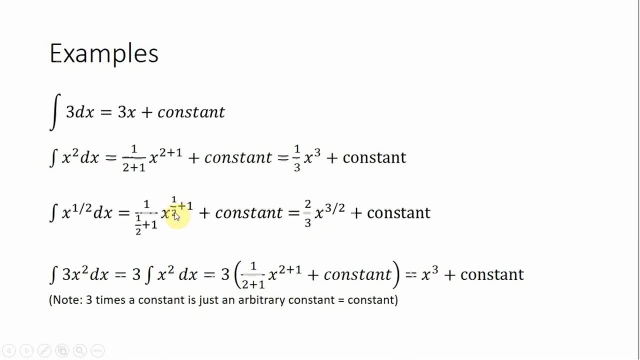 to be raised to one-half plus one And simplifying that all of this background, 특별그리지 over here is just two-thirds, One-half plus one is 1.5 or three-halves is two-thirds And we have our answer. 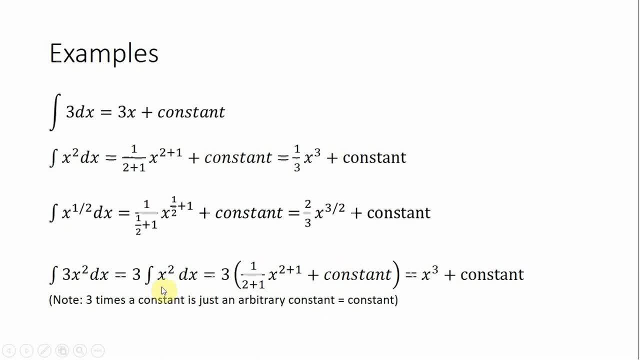 And let's look at: uh, I can bring the constant 저목 자� into the front. We're going to take the integral of 3x squared, bringing the threex squared out into the front, And then to put all of that solution together, you're going to take one-third, one-third, three-halves, three-halves And we're going to press it in the middle and slide it use to them to make this. 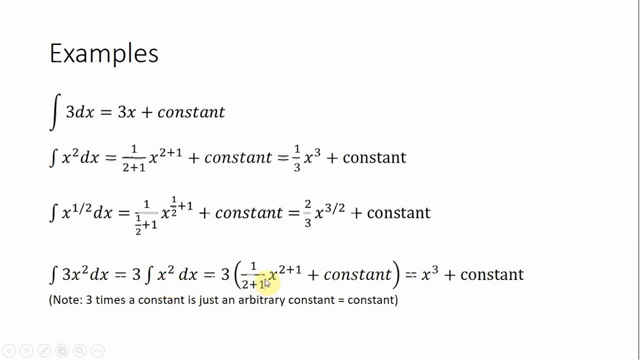 front, taking the integral of x squared, which we already saw over here. actually we have this, and that just simplifies to x raised to the third power. we got three divided by three, so all of that cancels to one. so we're just left with x raised to the third power plus some constant. 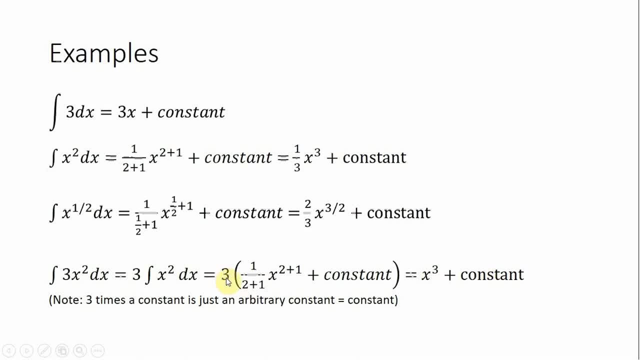 one thing to note here: this three is, you know, multiplied through by this constant, but that's really inconsequential. three times a constant is just an arbitrary constant. so I'm just calling it a constant, okay. so no big deal. and again, we could check our answer if we were to take the 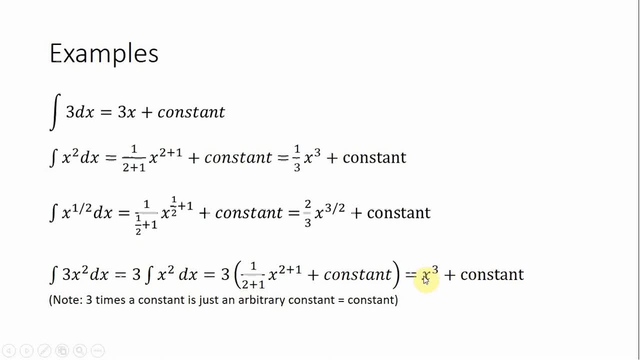 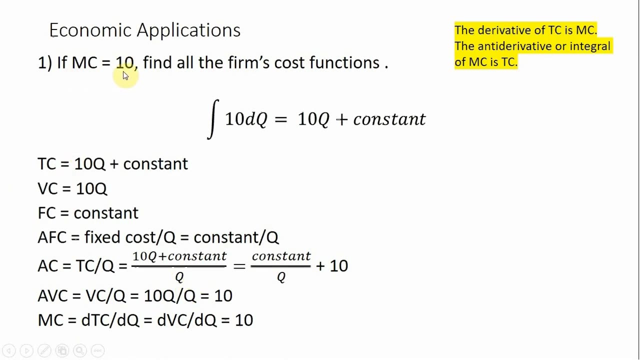 derivative of this result. down here we get 3x squared. derivative of constant is zero. so we get back what we're trying to integrate in the first place and now some economic applications. so here we have marginal cost, which we know is a slope function. the original function is total cost. so if you take the 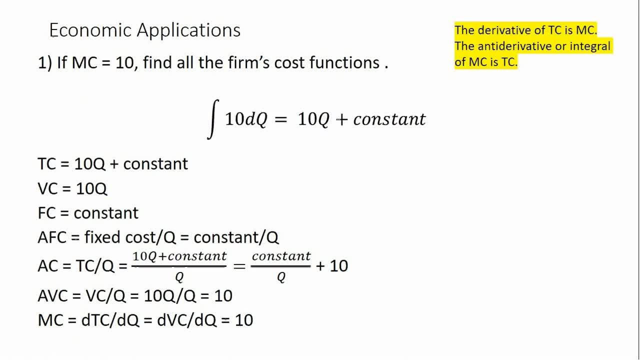 derivative of total cost, you get marginal cost. so now we're kind of doing the opposite, the anti-derivative. so we want to go from marginal cost to total cost and in fact what we'll do here we'll find all the firm's cost functions. so integrating 10 we get from our rules, we're 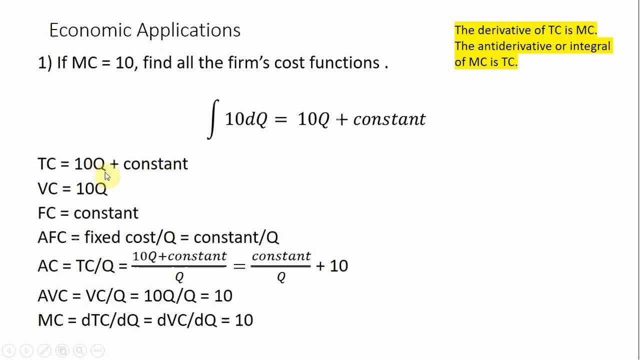 going to take our total cost. so that's what total cost equals. so total cost equals 10q plus a constant variable cost is just the part right here. 10q, this constant here is just fixed cost. if we wanted average fixed cost, we would take the constant or fixed cost divided by q. if we want to, 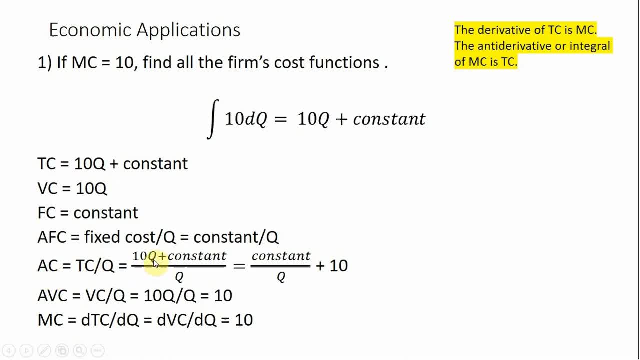 get average total cost, total cost divided by q. so 10q plus constant, all divided by q. simple, это simple applies to this. 10q divided by q is just 10.. If we wanted to get average variable cost, we would take the variable cost equation and divide it by q, which in this case would just 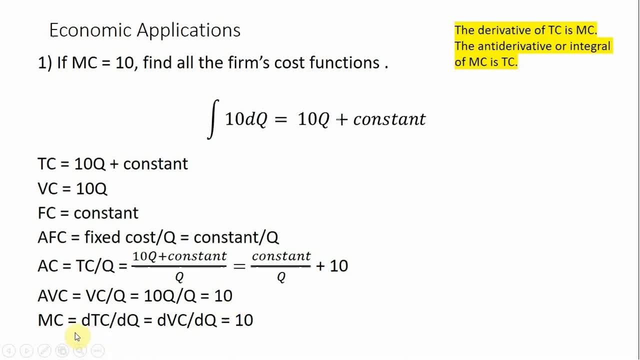 give us 10.. And again, we can double check our math here: If we take the derivative of total cost, we will get marginal cost, and that's just 10, and that's what we started the problem with. Alright, let's do a slightly more complicated marginal cost function Here. 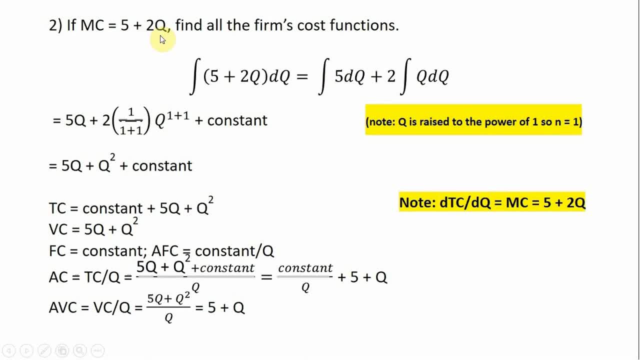 we're going to let marginal cost equal 5 plus 2q and, as before, we'll find all the firm's cost functions. So, taking the integral of 5 plus 2q, we're going to write it like this: I'm going to break this into basically two functions, the 5 and the 2q. realizing: 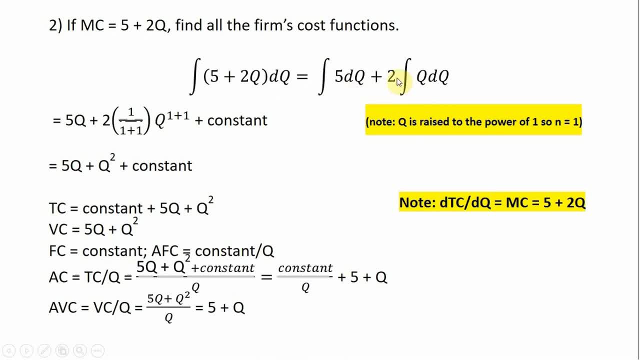 we can bring the 2 out in front of the integral sign here for the 2q part. So the integral of 5 is just 5q, The integral of q, and again following that rule- note here- q is raised to the power of. 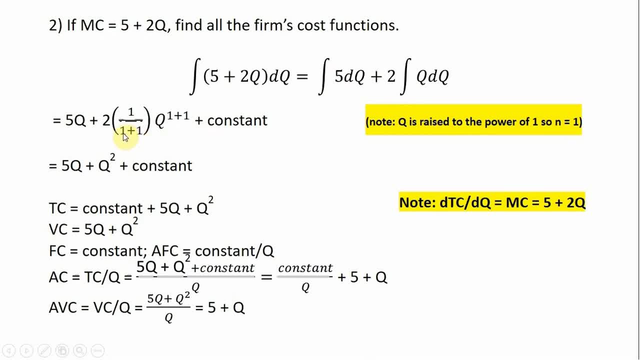 1, so n equals 1, so we got n plus 1, where n is 1.. And again, following that power of function rule, n plus 1, where n is 1, it's going to all equal this, And that will very. 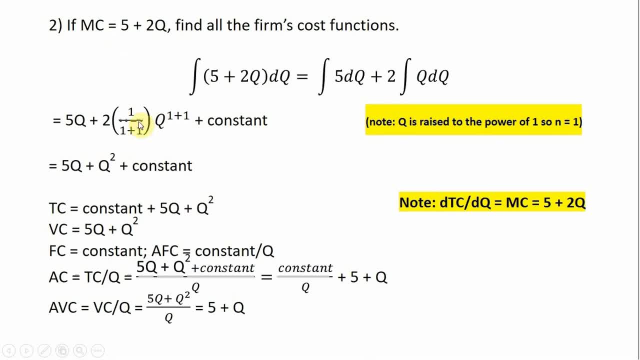 nicely simplify to just q squared. So we've got 2 divided by one half q squared. so simplifying it down here, that now becomes our total cost equation. So total cost is a constant fixed cost plus the variable cost part. So variable cost is 5q plus q squared Fixed cost. you know before nothing too. 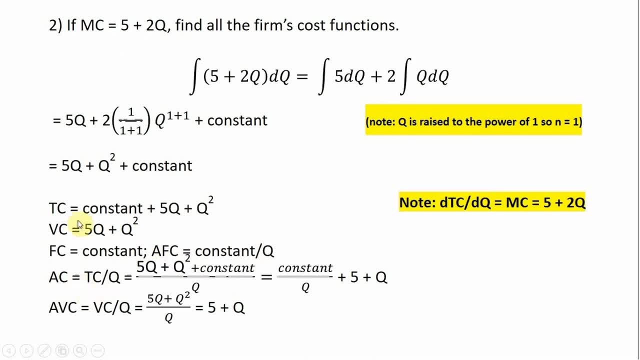 interesting here: Average cost, just taking the total cost equation that's going to be, I don't know, one, two, three, four, five, six, seven, eight, nine, 10,, 12,, 11,, 12,, 13,. 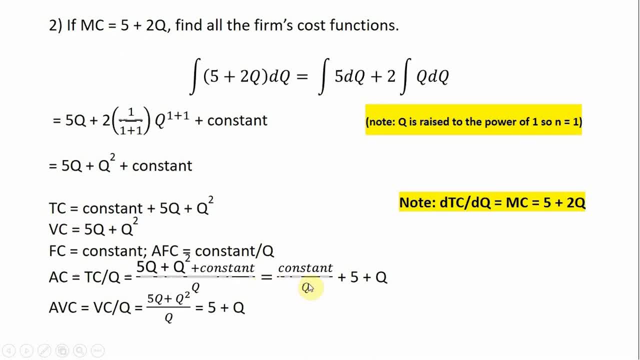 12,, 13,, 13,, 14,, 14,, 15,, 16.. And then we have the variable cost, which is going to be 5q plus, and dividing it through by Q simplifies to something that looks like this: 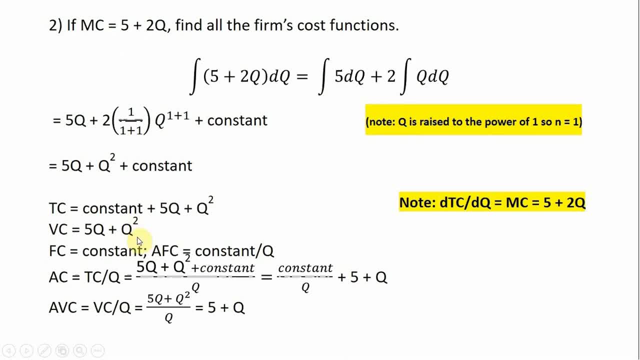 Average variable cost. just taking the variable cost equation and dividing it through by Q, we get something that looks like this, And again, note here- marginal cost. if we were to take the derivative of total cost, you'd get 5 plus 2Q, and that's what we started this problem with. 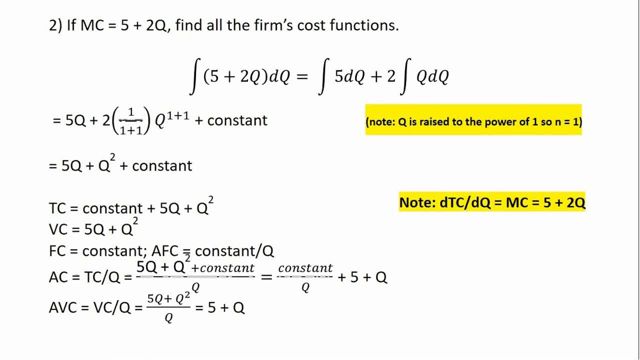 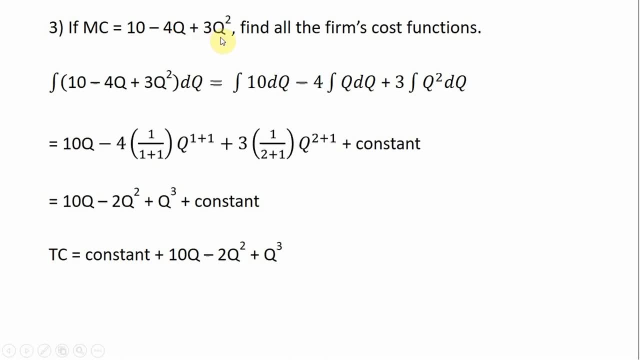 All right, and a slightly more complicated marginal cost function, which will be our last example. Marginal cost equals 10 minus 4Q plus 3Q squared. From here we're going to integrate it, get the integral to find total cost and then go from there. 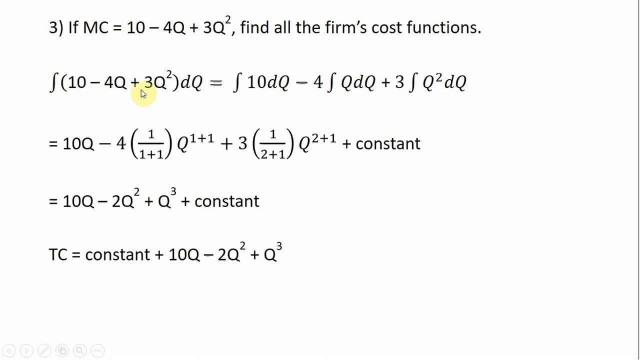 So first writing the integral of 10 minus 4Q plus 3Q squared. breaking this down into, you know basically sums and differences. So we got the 10 part over here. We got the Q over here. I brought the minus 4 out in front of the integral sign. 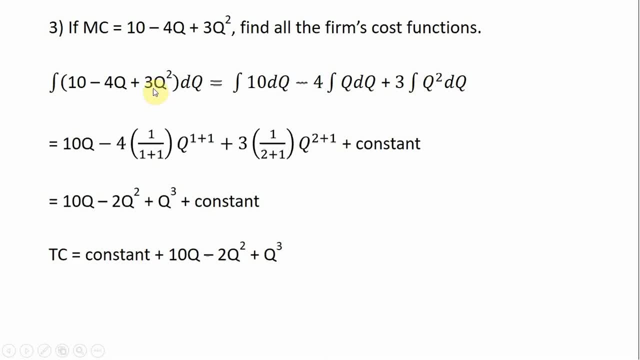 We got the Q squared over here And again. the one rule allows us to bring the constant out in front of the integral sign, so we do that. So the integral of 10 is just 10Q. The integral of 4Q is going to be given by this. 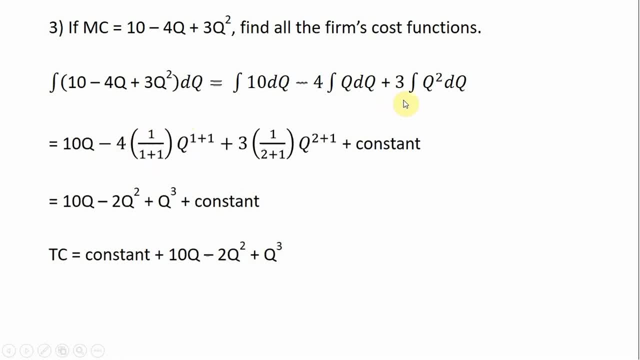 Okay, so we're going to get that, And then the integral of 3Q squared is going to be given by this, And we're going to just add on a constant here at the end And now simplify. So 10Q, 10Q. 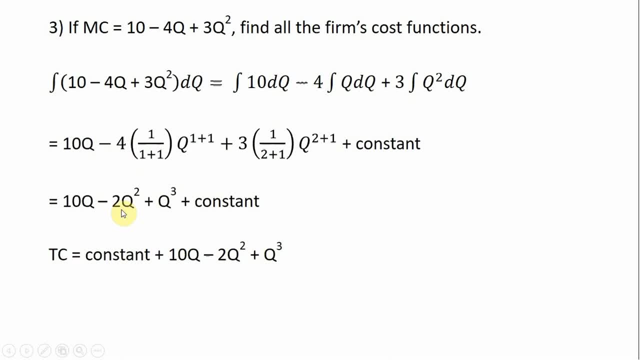 We got minus 4 divided by 2.. So that's minus 2Q squared. We have 3 divided by 3.. So that's just 1.. And then we got Q raised to the power of 3.. And then the constant. 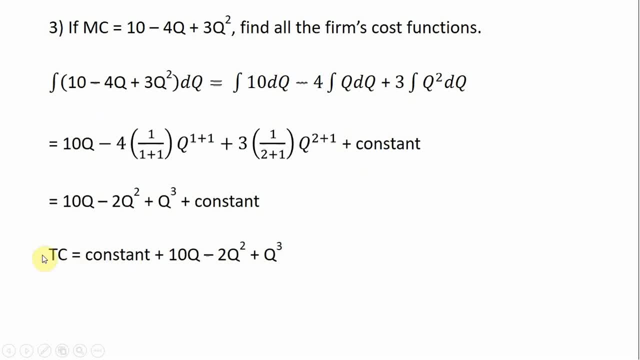 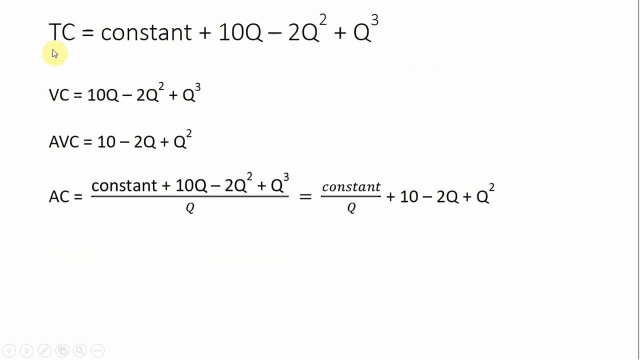 So this total cost. so from marginal cost we go to total cost. It looks like this: And then on the you know, getting the remaining cost functions. I didn't do fixed cost or average fixed cost. That is basically unchanged from all the other examples.